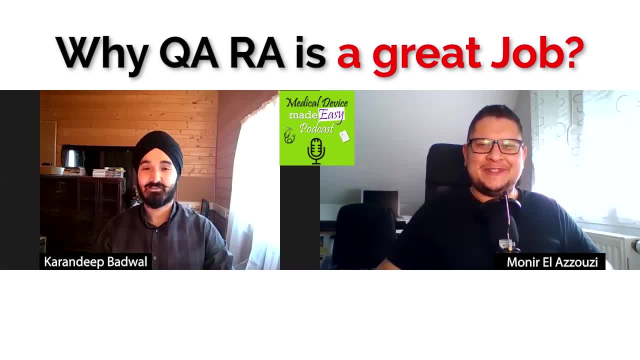 Welcome to the Medical Device School. So this is a bonus episode about the Medical Device Made Easy podcast, And today we'll talk about quality and regulatory affairs and specifically why a quality and regulatory affairs job is a great job, And for that I have with me Karan Deep Badwal. So Karan 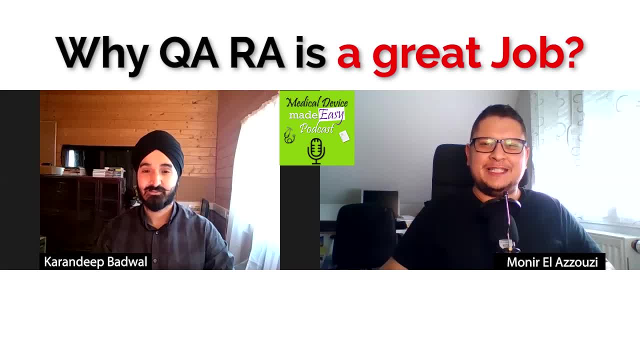 Deep was with us on episode 31 of the Medical Device Made Easy podcast, where he tried to explain to us how to enter the regulatory affairs field. So, Karan Deep, welcome back to the Medical Device School. Thank you for having me back, Manier. It's a pleasure to be back here. So, as we said, 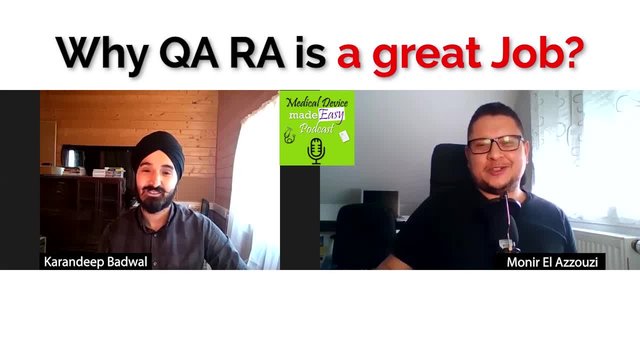 so let's try to explain, or let's try to say to people why quality and regulatory affairs is a great job. So can you start and tell us more about your journey and why you think that this is a great job? Yeah, I mean quality and regulatory. unfortunately, it has one of the worst reputations. 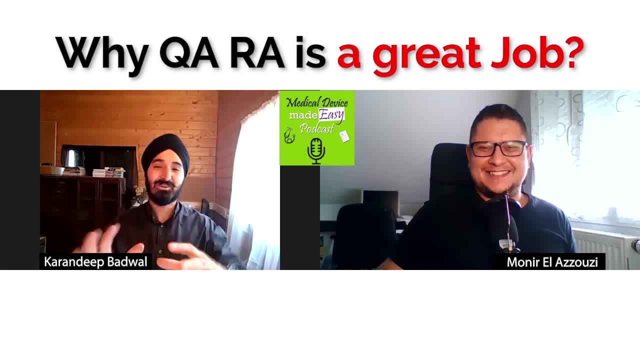 because in most sort of companies, we're always the guys that stop. you say no, you can't do this, This is the way You need to do it, But quality and regulatory affairs. it's a brilliant job because, unlike R&D. 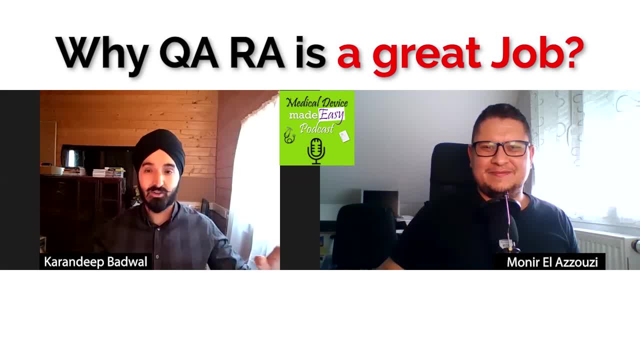 and other departments that may be out there. you have a top line view of the company. You get to see each and every aspect of the company and how that fits into the quality system. obviously, whether that be through your risk assessments, whether your technical files, you know everything. 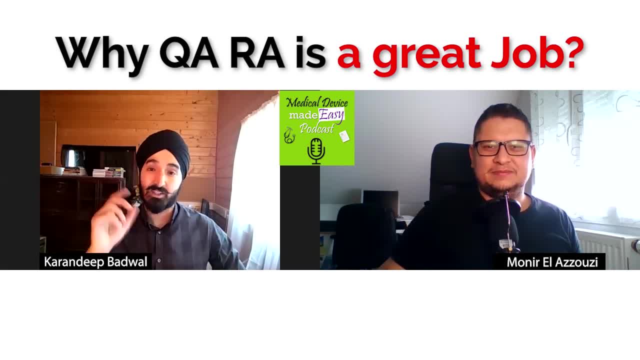 about the products And you are in the perfect position to make sure that the product number one is of the best quality and the process and the quality management systems are the company as best as it can be. So if you are an individual who's sort of hardworking, you're not going to 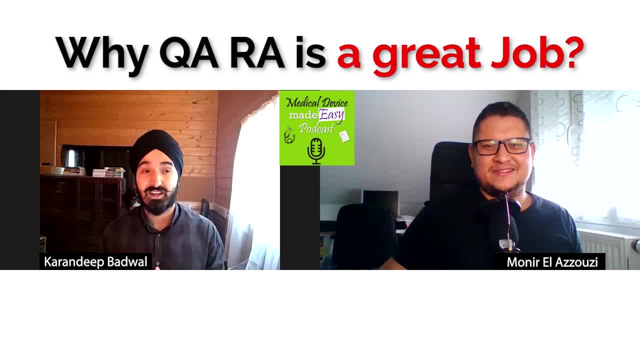 be highly organized. you'd like to have a lot of control and you know you want to sort of have a high level of maintenance in your role. quality and regulatory is one of the best roles you can ever have in the medical devices industries for that. So mainly what we from my side. so when I was on 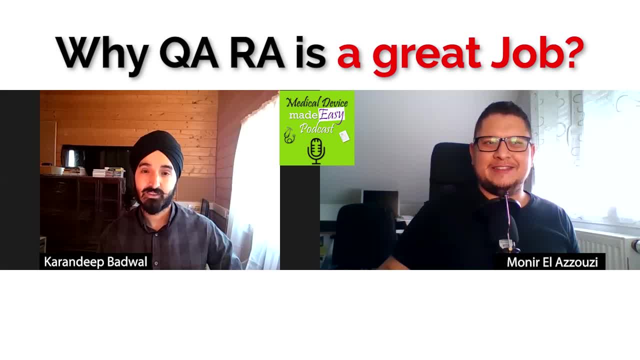 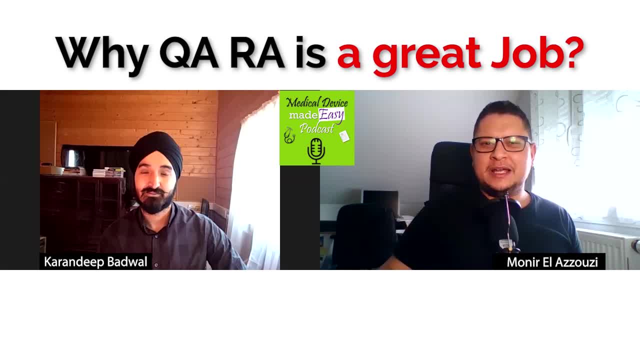 this kind of thing, And I had the chance to have really a good mentor, because when I was looking for an internship I didn't find anything, and I found only something with quality and regulatory affairs, So I had to do it anyway. So I said, okay, let's do it, And I had really a great 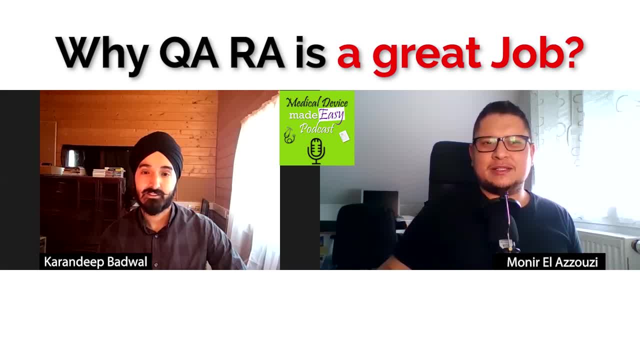 mentor. that showed me really that, as we said so, quality and regulatory affairs is really overseeing the whole company. They are the law of the company, They are building the law, They are making the law applicable, et cetera, et cetera, which is really something that 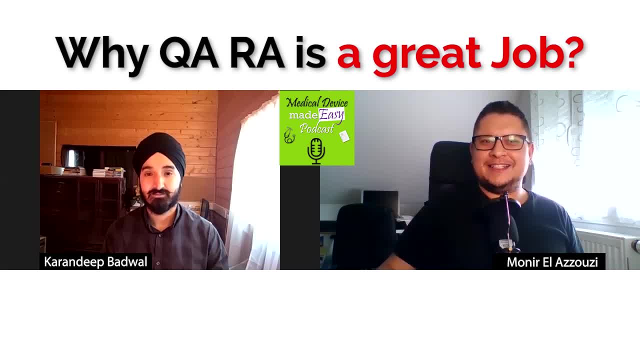 was really exciting for me to say, oh really, I have to audit those people to check they are doing a good job. I have to tell on the procedure what they should or should not do and how they should do it, et cetera, et cetera. So it was really great. Not on the way that I have the 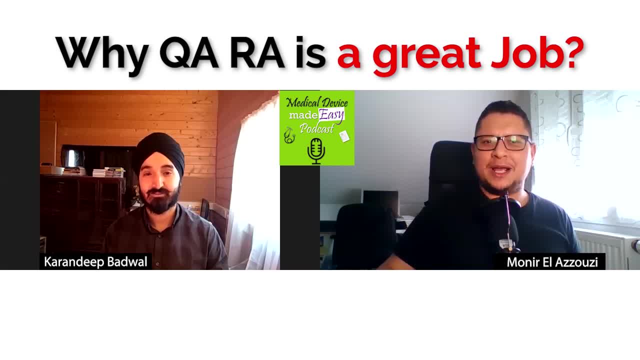 power. It's more on the way that I can help people and I can make them do the right things from the beginning. But you said also something that's interesting is why it's also something that maybe people hate. So it's quite it's like similar to what you. 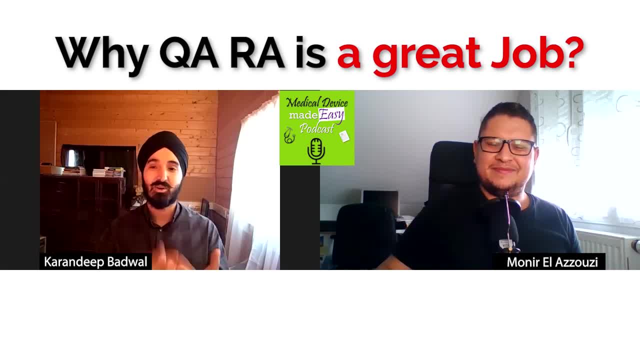 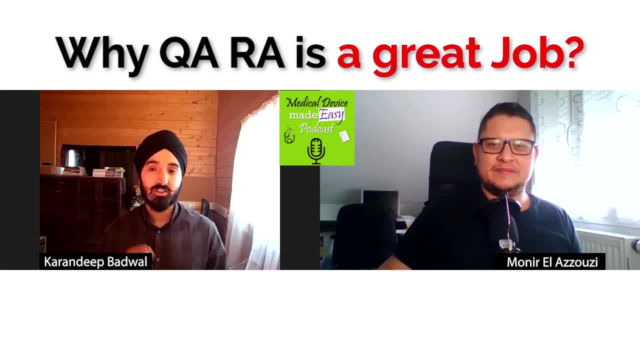 is they simply don't understand what quality and regulatory affairs is. So what I've always done in every single job that I've gone into, I've always made sure that I spent time in other departments- whether that be labs, R&D- to show them the importance of quality and what it's all. 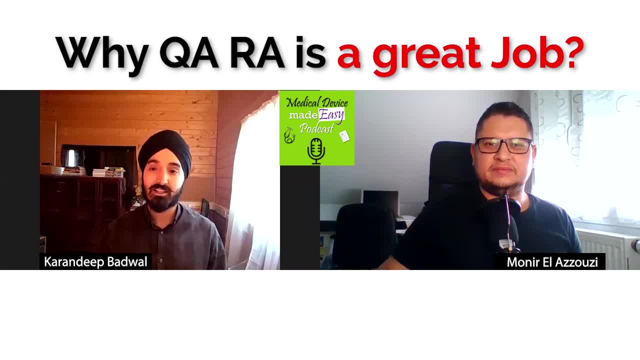 about. I would show them copies of the standards. And once they gain that understanding as to why we do this and by doing these sort of things we can have the best quality product out there- They begin to change their way. So they understand, say, oh, I know why I'm doing this. 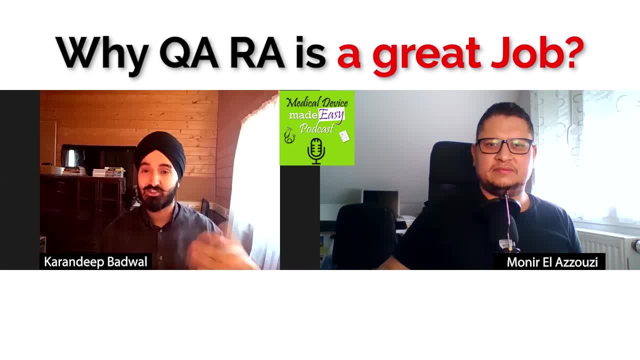 paperwork is for traceability, So if something goes wrong, I can go back, I can check my work And we have all these procedures in place, And that's basically. it's about changing the understanding of the individual, And it's at that point they begin to stop hating you. So I've 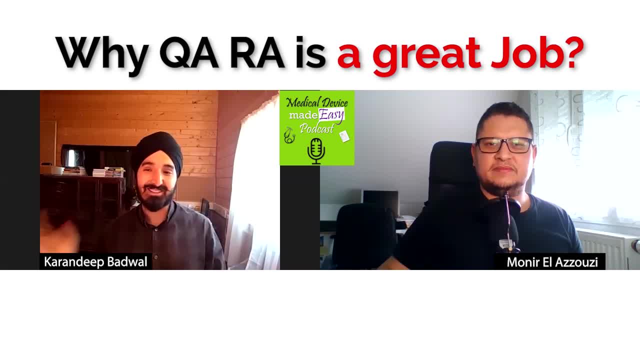 always made sure that whenever I've gone into a company, I'm not the individual to be hated. I'm the individual to be liked, because I'll change the perspective of what it's actually about, And it's mainly the. that's what. what is interesting is the fact that 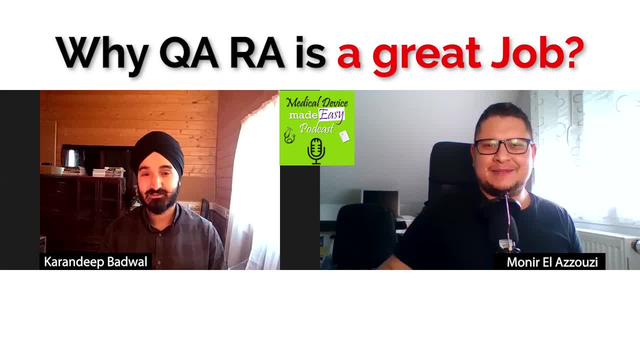 it depends on your kind of mindset. But yeah, there are people that can really hate quality because of some wrong mindset on the on the quality departments, or can love it because they really see that those people are not here to just point out the wrong things, but also to help. 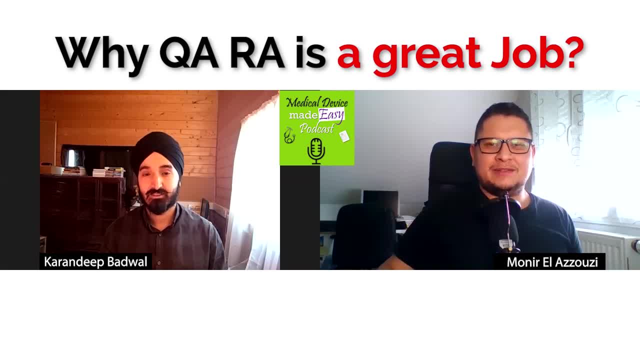 them to do the right things, which is something that is that is for me, if I can say, really really interesting. So now that we have cleared that, really quality and regret your face, a great job. So I mean, I hope people really understood that. So is there some kind of skills or things that people have to? 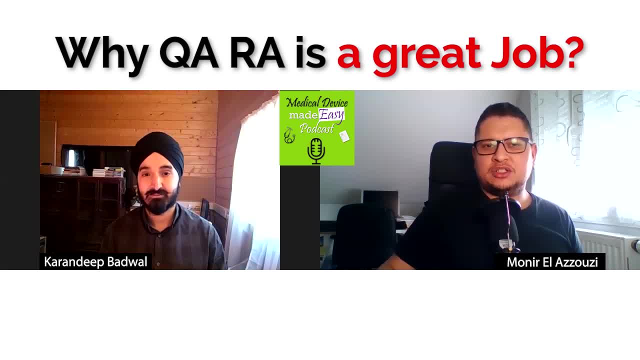 have, if I can say, to really love this kind of position. Yeah, I mean, the first thing is you have to be a very disciplined individual. you know, whatever it may be, you need to make sure you do it properly. you can't cut corners. 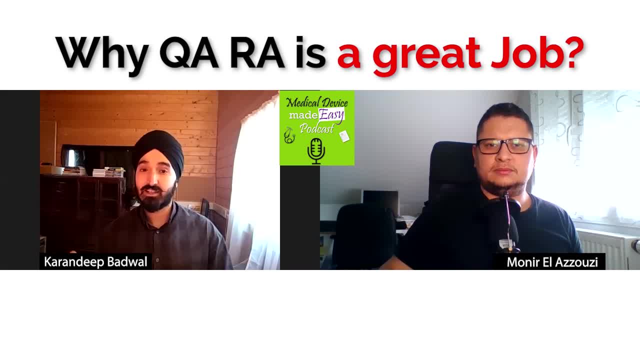 and you need to make sure that you invest the time into something. There's a saying out there: if you do not have the time to invest it now, when would you have the time to fix it? So invest the time, do it properly the first time. So, number one: you need to be disciplined. 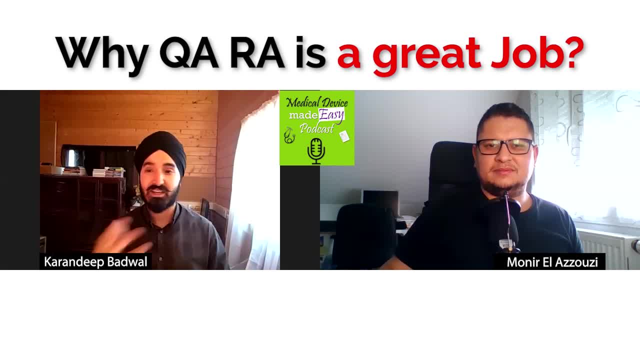 Number two, of course, is being well organized. you know quality standards are changing: MDD, MDR. for us guys here in the UK- Brexit- all these different things are going on all the time, So you need to make sure that you stay on top of those different things as well. 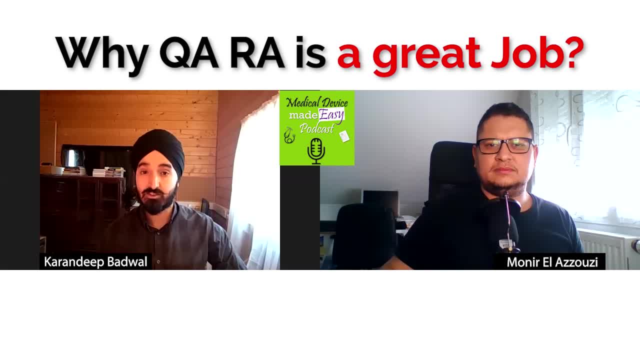 And number three is you need to make sure that you have good communication skills. I mean, you can put all the policies and procedures in place within the company But, like I said, if the workforce don't understand it and you're not communicating that out properly, then 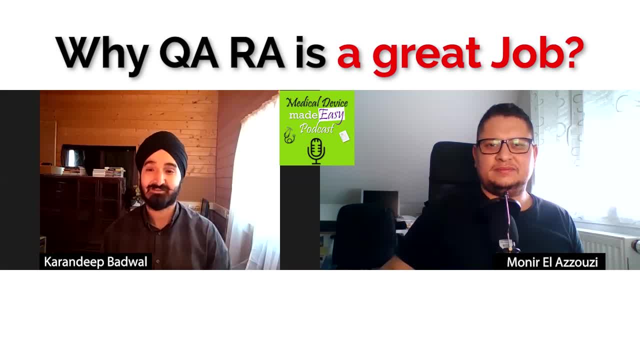 quite frankly, you're not going to be able to do it, So I think it's important to be disciplined. No one's going to follow what you put into place Exactly, And it's really. the danger is the fact that you have a procedure where it's written that 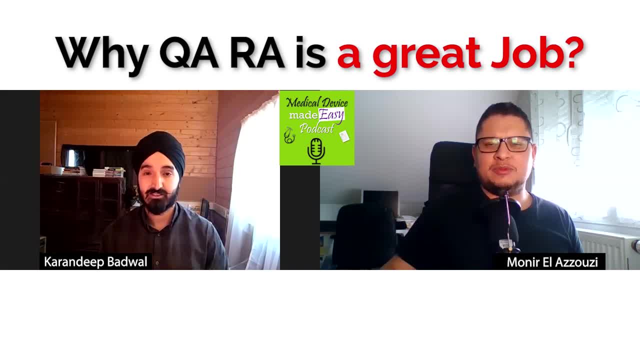 you should do this and you are not executing that because, mainly, you are in disagreement about it, And it's what I'm giving as an advice to people that are writing procedures is: write what you do and do what you write. So mainly, don't put things additional, things that you are. 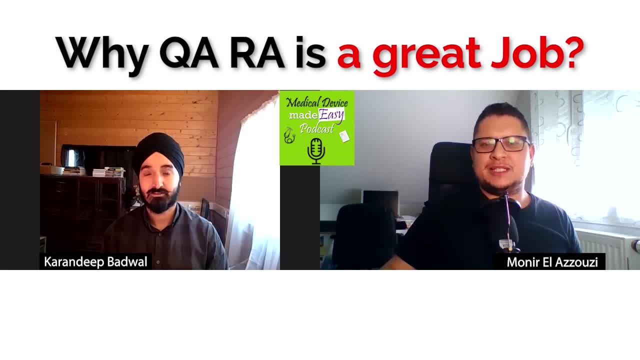 sure that nobody will follow, just because you think that, because it's written, they will follow it. So it's really also an important thing. Okay, something else from your side. Yeah, I mean, hopefully I've changed your view on what quality and regulatory affairs is. I mean.